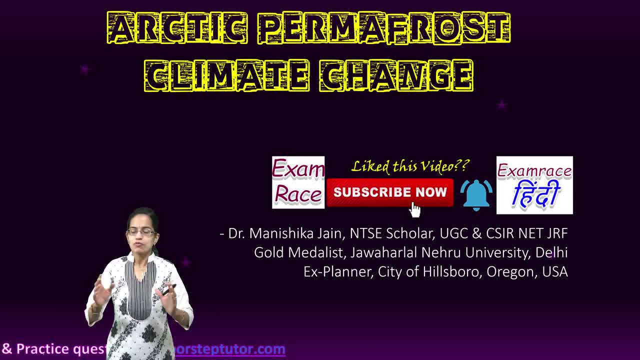 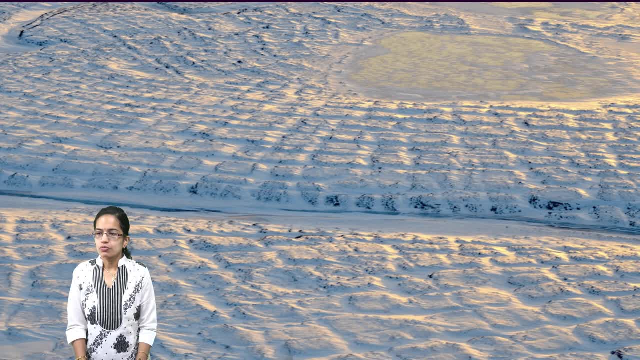 Climate change and arctic permafrost. So before we begin with this topic- a very, very important and relevant topic for today- we need to understand what is permafrost. So permafrost is nothing but a permanently frozen layer that can be seen, and this frozen layer is 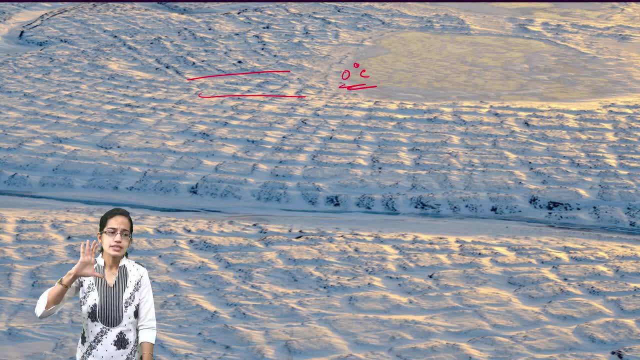 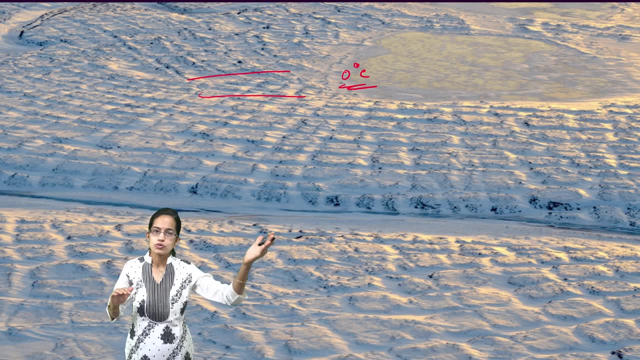 at nearly zero degrees and has miles of thickness. It is including high mountains, the earth's higher latitude areas, mainly the north pole and the south pole, and covers a huge proportion of earth. Now understand that if this ice suddenly starts to thaw or melt, 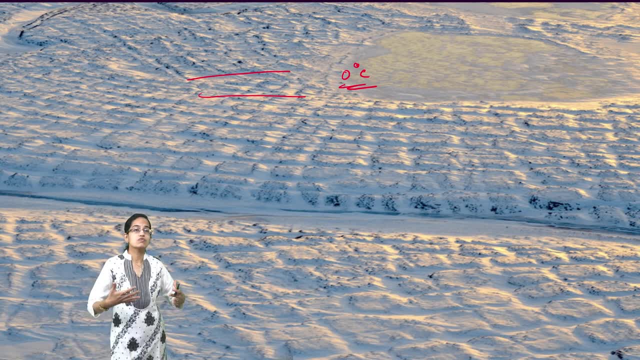 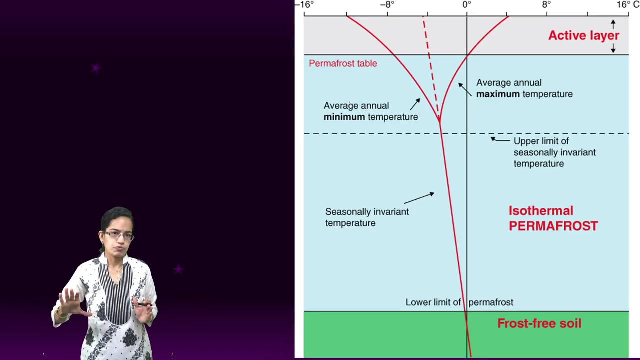 what would be the scenario? A large amount of region would be covered with water, or we would say, would be flooded. So how do we understand this permafrost, What are the layers within the permafrost and how we see the development if this permafrost starts to thaw all of the sudden? Now let's understand the structure of permafrost. 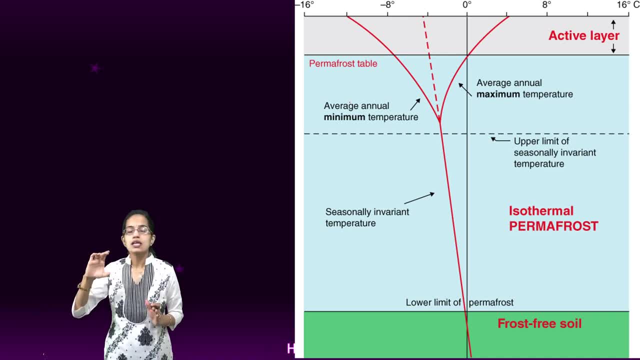 Permafrost has three important sections. The first is the layer of active permafrost. The active permafrost is the layer which is the topmost layer and it does not stay frozen throughout the year. During the warm months it melts and during the winter months it starts to freeze again. 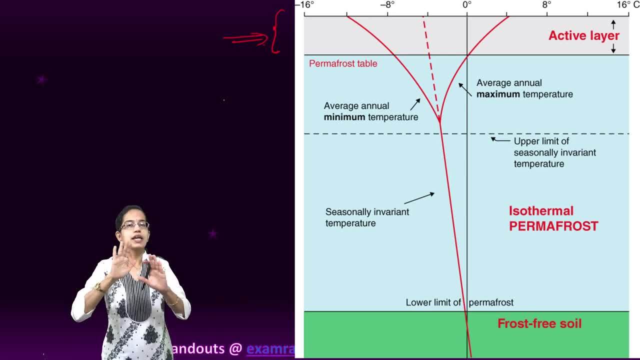 However, in extremely cold area it rarely thaws, So it rarely melts. in simple words Now, the layer below this is what is known as the permanent permafrost. This is the layer which is a mix of soil and minerals and remains permanently frozen below the active layer. and within this layer we have 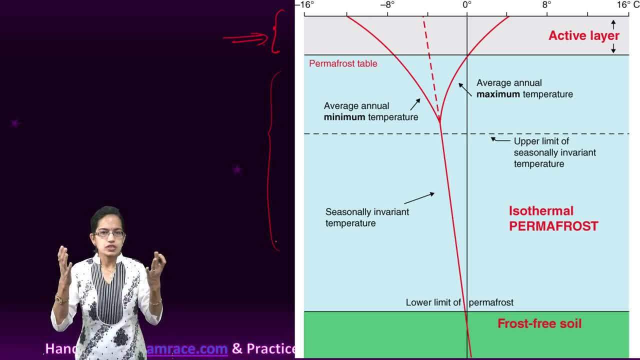 ice wedges that are seen. So permafrost. if I give you a overall aspect about it, it is a composition of ice with soil, rock, minerals and some of the dead animals and plants that are there. All this are part and composition of the permafrost layer. Now, while recently active, 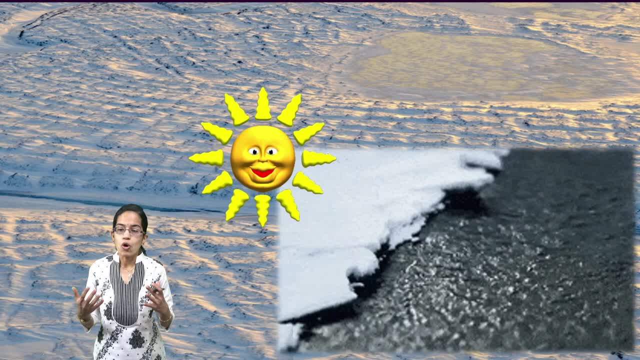 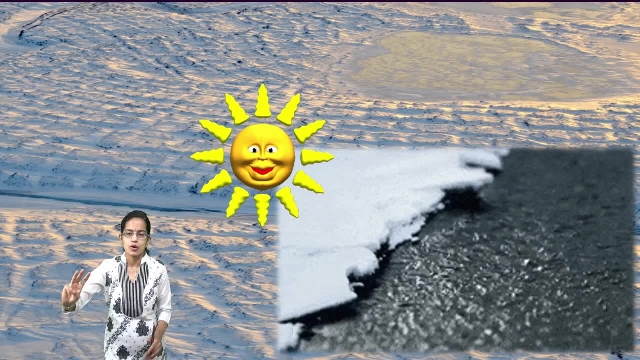 permafrost has come into light and the thawing of the arctic permafrost has created an important concern for humanity. There are three important reasons cited for this. The first is when you have sun rich permafrost. motivo que sólo il banyak ne Hotelo. First is when you have sun rich permafrost. The second is when you have sun rich permafrost blocked through the cold. photographer reminds us of permitiru, queen country��ի size, a lingi eficencia Есть, ㅋㅋㅋㅋ. более cakey to look at this pillow. 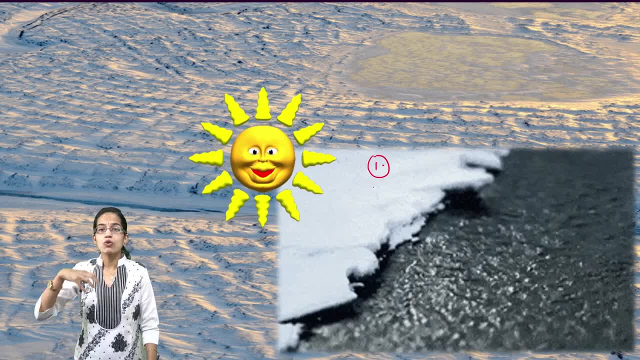 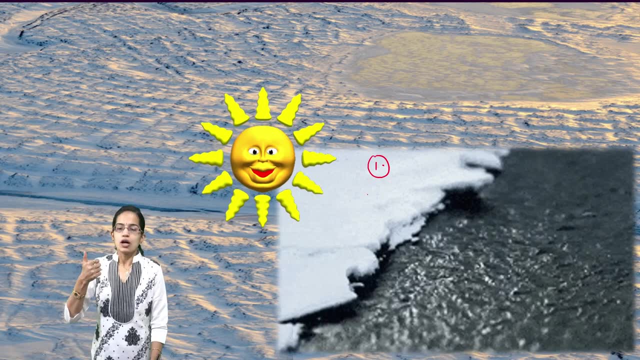 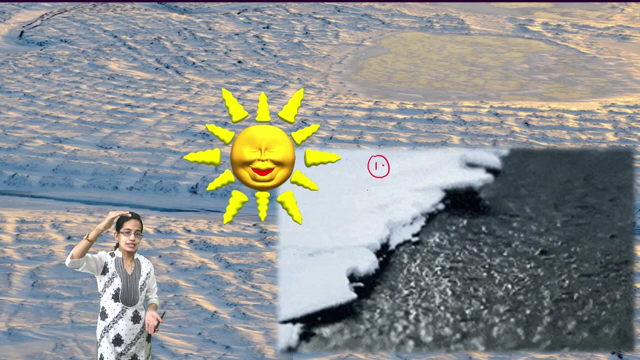 is falling onto the polar areas. we are specifically focusing on arctic regions right now because we have a lot of dwelling in and around those areas. now, when this arctic permafrost starts to thaw, what would happen, since it is miles of ice that is there? there are numerous homes and livings. dwellings that are being built on the permafrost area. so what would happen if this ice suddenly starts to thaw? if this ice suddenly starts to thaw, many of the villages that are located in the northern boundaries would be destroyed: the roads that have been constructed, the infrastructure. 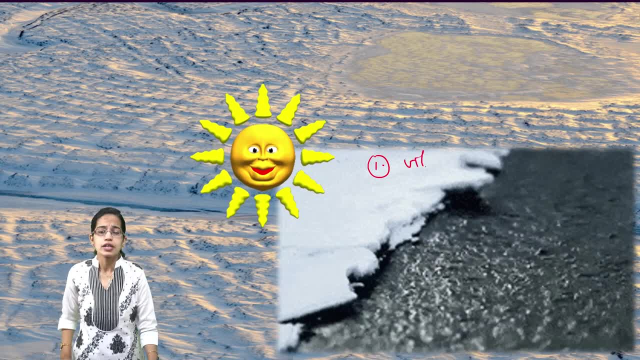 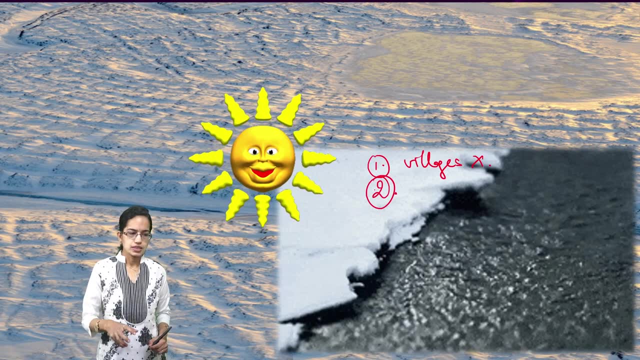 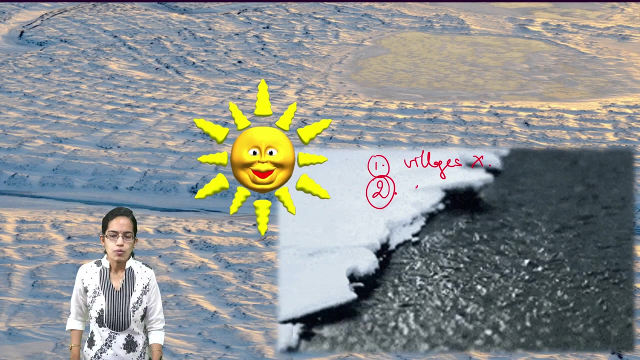 that has been laid down would be destroyed. so destruction of villages would be one of the first concerns that would be there. the second important concern is when the permafrost is frozen, the plant material is in the soil and this is in the form of what it is in the 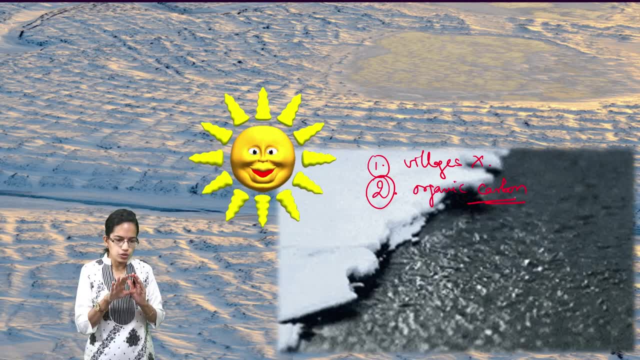 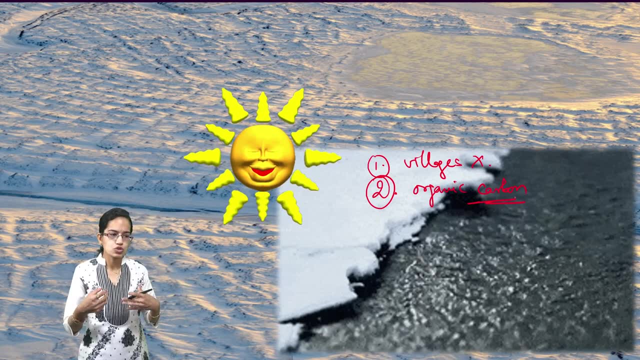 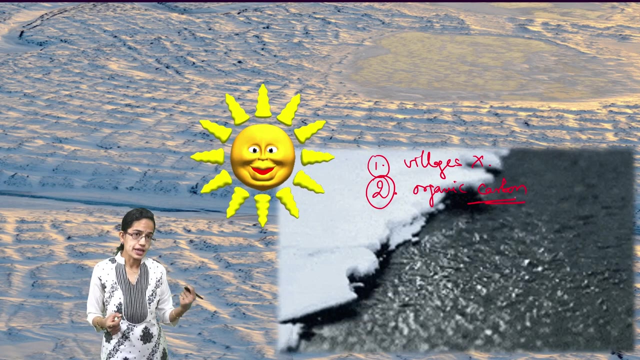 form of organic carbon. now it cannot decompose. since it is cold, it cannot rot away. but as soon as the permafrost begins to thaw, what happens? the microbes start to act and they start to decompose the material. once the microbes start to decompose the material, this would 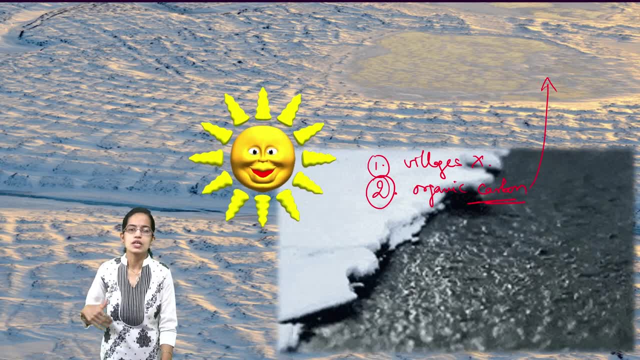 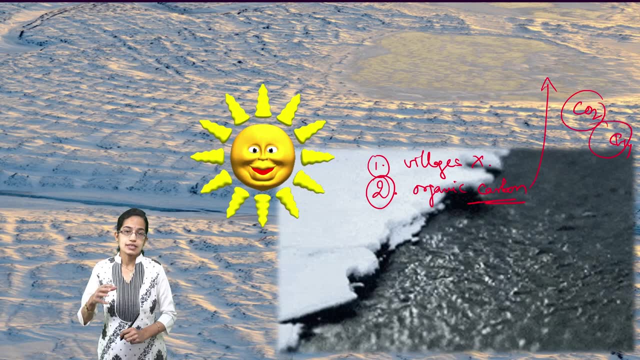 relieve the release this carbon into the atmosphere, and this would be in the form of methane and carbon dioxide. So those would be the materials that would be in the form of carbon dioxide, and then those would be the gases, the greenhouse gases, that would be emitted into the atmosphere. 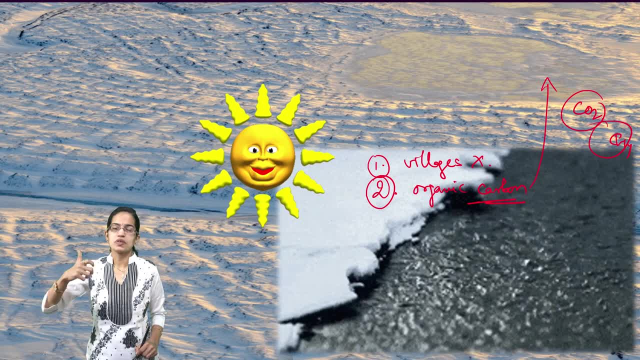 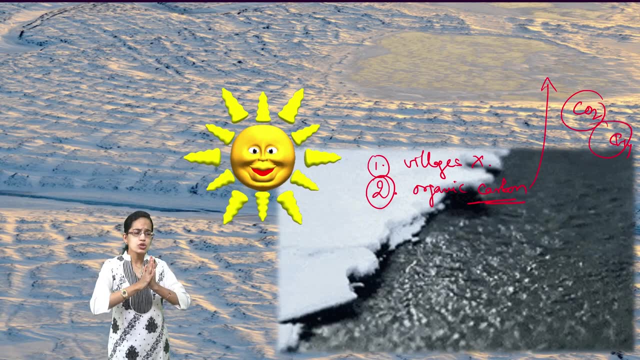 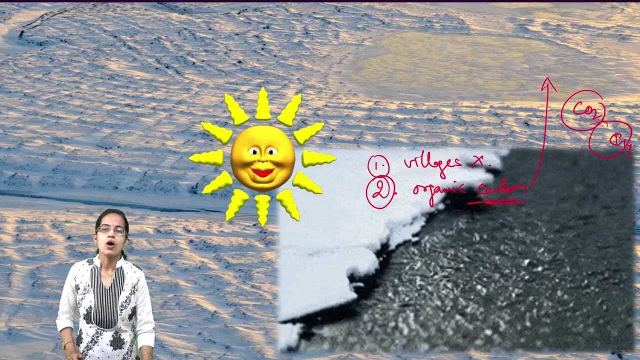 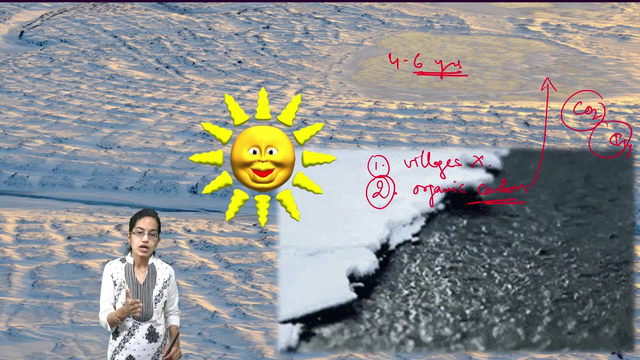 now, since these greenhouse gases would be emitted into the atmosphere. it would lead to climate change. the studies have cited that there is a huge amount of carbon that is seen, and the studies revealed that if the permafrost starts to thaw, there would be around four to six years of carbon that would be released into the atmosphere. however, what the findings?